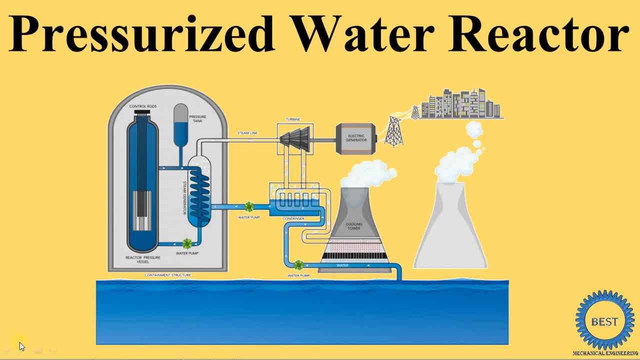 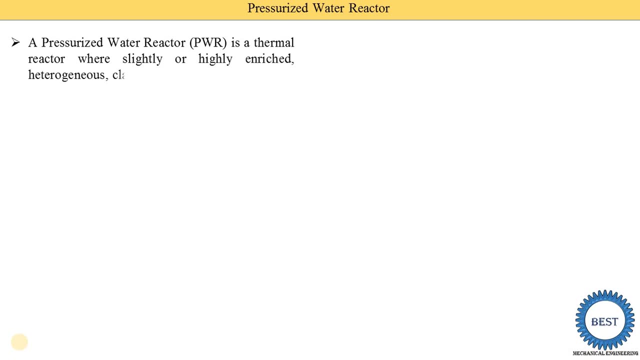 In this video I explain construction, working advantages and disadvantages of pressurized water reactor. First I explain the construction of the pressurized water reactors. So first we discuss about the which type of the fuel and which type of the reactors and which types of the moderator is used in a PWR. 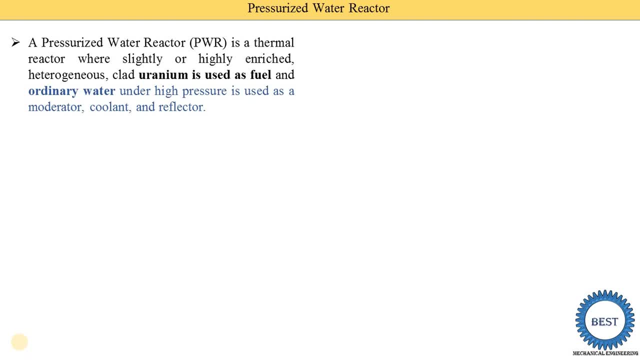 PWR means pressurized water reactors. In a PWR, highly enriched uranium is used as a fuel And the reactor is heterogeneous. Heterogeneous reactor means the fuel rod is surrounding by the moderator. It is called as the heterogeneous reactors. 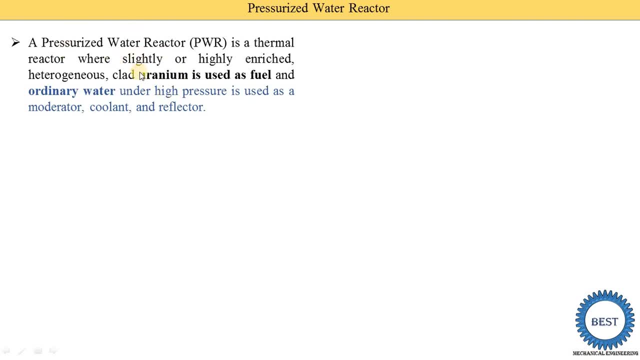 And this uranium is clad. uranium And ordinary water under high pressure is used as a moderator coolant and reflector Means. Ordinarily, water is used for moderators, coolant, as well as for the reflectors. Now, here you see. this is the diagrams of the pressurized water reactors. 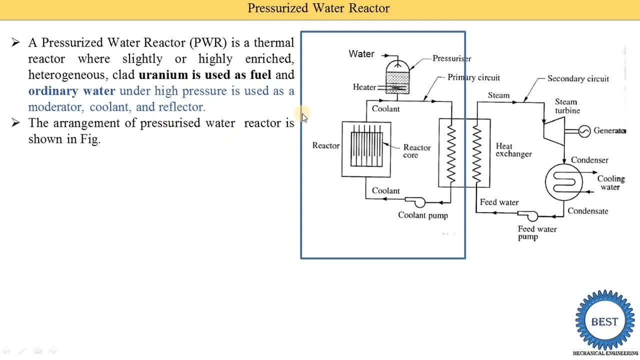 Or a arrangement of pressurized water reactor in this diagram. So these PWR reactors are divided in a two circuit. One is called as the primary circuit. So here in this rectangle You see, it is called as the primary circuit And this part is called as the secondary circuit. 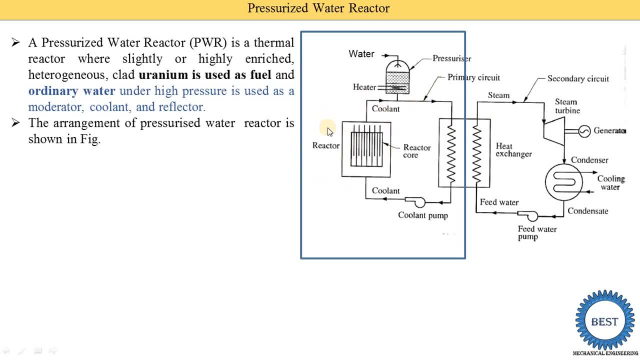 And in this primary circuit, what are the component is there? First one is this reactor. These are the pressurizers And this is the heat exchanger And this coolant pump. This is the secondary circuit, That is the steam turbine condenser pump and this heat exchangers. 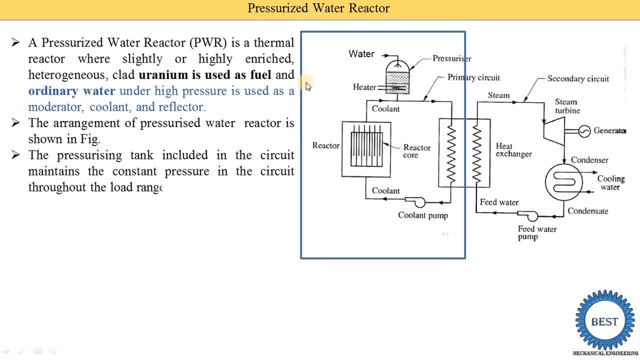 Why its name is given the pressurized, Because this pressurizer is used in this primary circuit. That's why its name is given the pressurized water reactors. Now, what is the functions And what is the constructions of this pressurizers? 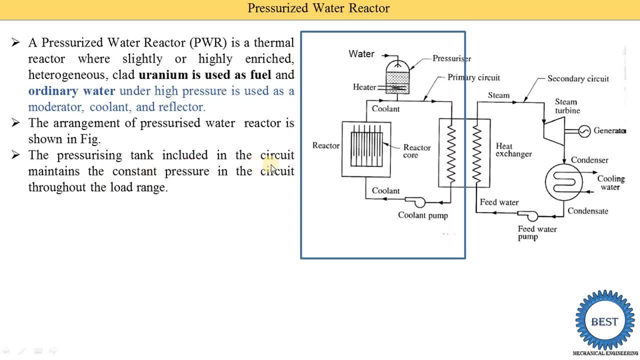 The pressurizing tank include in the circuit to maintain the constant pressure in the circuit throughout the lower range Means. The function of this pressurizer is to maintain the constant pressure in this primary circuit. So this is the pressurizers, And this pressurizer is consist of this heater and the vessel. 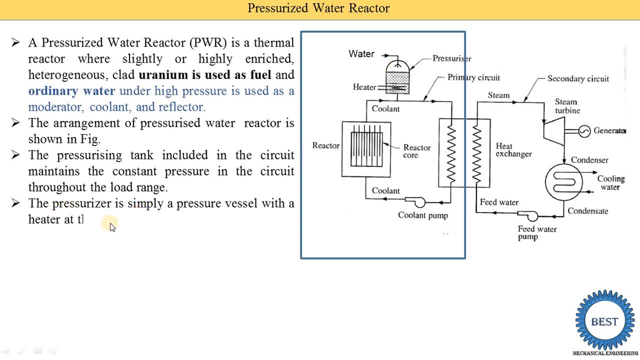 Means this outer part is called as the vessel. The pressurizer is simply a pressure vessel with a heater at the bottom and the water is spray at the top, Means at the bottom of this pressurizer. here you see, one electric heater is putted. 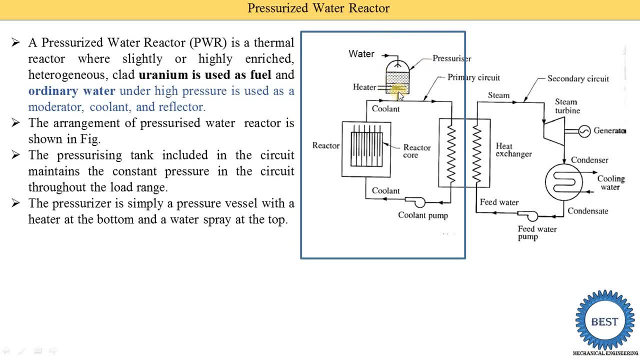 And from the top the water is spray. So this is the construction of this pressurizer, or a pressurizing tank. The water in the pressurizer is boiled and converted into the steam by electric heating coils. Before starting the reactors- Means before starting the reactors- we need to start this heater. 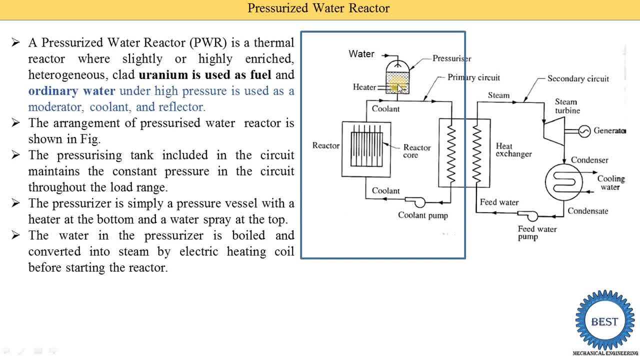 And this heater is boiled the waters And this boiled water is create the certain pressures in the primary circuit. So this result in a increase in the pressure Means. when we start this pressurizers, they increase the pressure in the primary circuits. If the primary circuit pressure become too high, 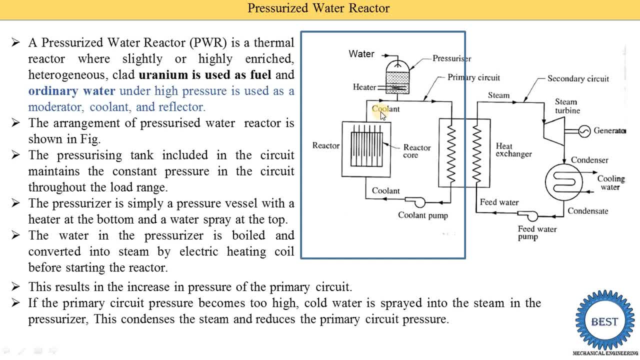 Means. it is not necessary, it is only increase the pressure. Sometimes the pressure is too high, Increase too high, Then we need to reduce the pressure. So how we are reduce the pressure So at that time we can spray the cold water. So cold water is spray into the steam. 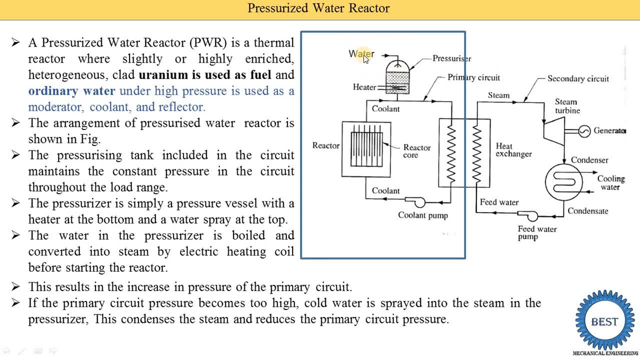 So here you see, in the upper parts of this pressurizers, the water spray is provided, So water is supplied and water is spray into the steam. So when we spray the water into the steam, what happens? They condense the steam Means, the steam is convert into the water. 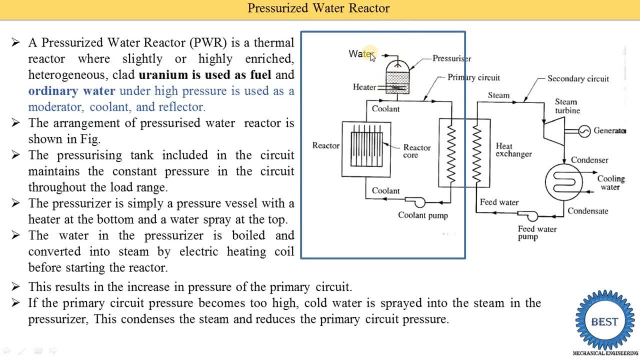 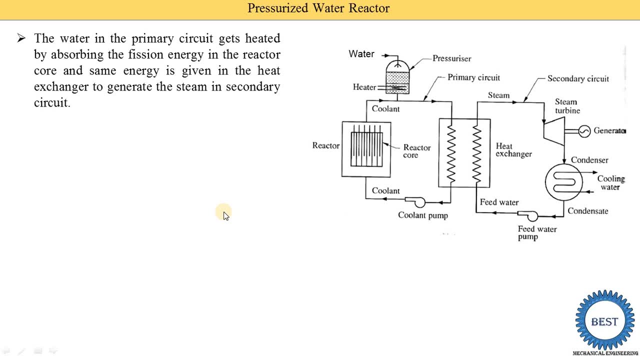 It is called as the condense the steam And reduce the pressure. Pressure in the primary circuit Means this pressurizer is used to increase the pressure or reduce the pressure. Ok Now, Now we understand its construction, Sorry. Now we understand the working of this PWR. 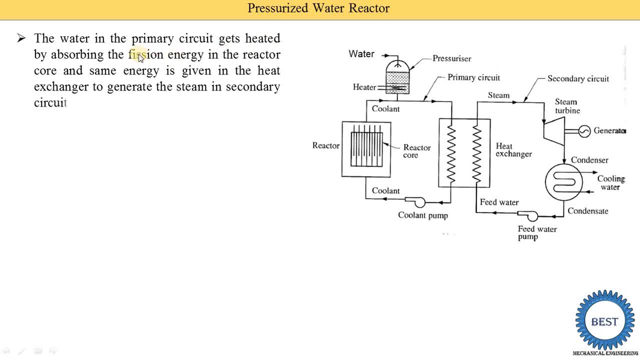 So water in the primary circuit get heated by absorbing the fission energy in the reactor core. So here you see, This is the reactors, And in the reactor the fission process is carried out And due to this fission process the heat energy is released. 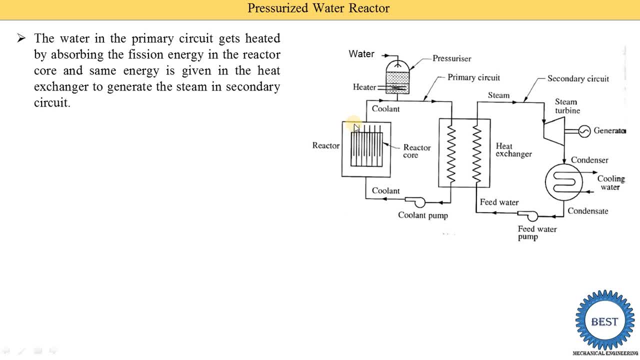 So this heat energy is absorbed by this coolant, Ok. So here you see, this coolant is enter into this reactor And in this PWR we are use the ordinary water as a coolant Means. the water is enter here, Ok, And this water is absorbed, this heat energy and this water is coming out. 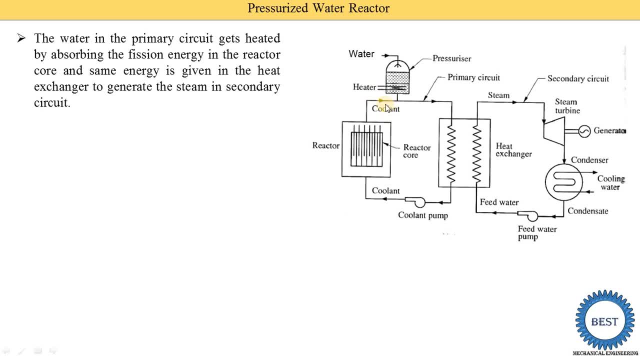 Ok, Why here water is coming out. We are not mention here the steam is out, We just mention this coolant is out. Because here the pressure is coming out, Because here the pressure is too high, That is, a 130 bar to 150 bar pressure are there. 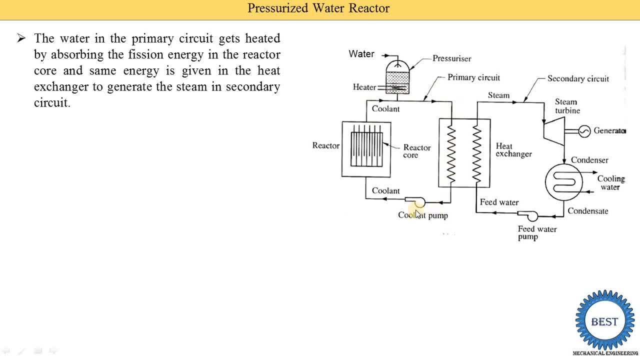 Ok, So here, only in the primary circuit, this water is circulate. No steam is there. Ok, Then after this water coming out from this reactor is supplied into this heat exchangers, Ok, And this heat exchangers, This water of the primary circuit, is supplied heat energy to this water of the secondary circuit. 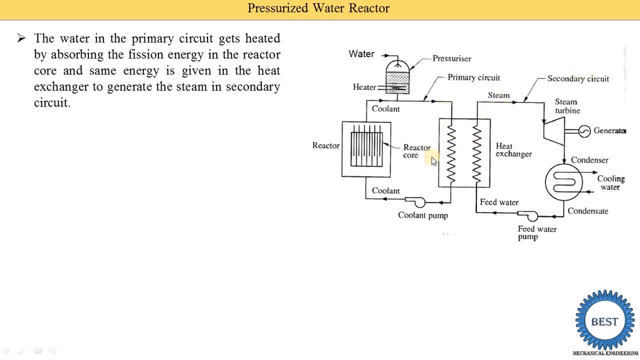 Here you see, This is the heat exchanger. are there Once heat is exchanged between the two medium? One medium is the water in the primary circuit and second medium is the feed water in the secondary circuit. Ok, So this feed water is converted into the steam here. 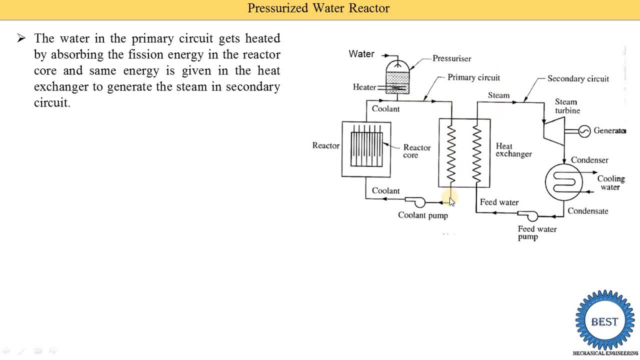 Ok, And in this primary circuit temperature of the water is reduced, Then it is supplied to this coolant pump and then again supplied to this reactors. So in order to prevent the boiling of water in the reactor core, it is keep under a pressure of about 130 to 150 bar. 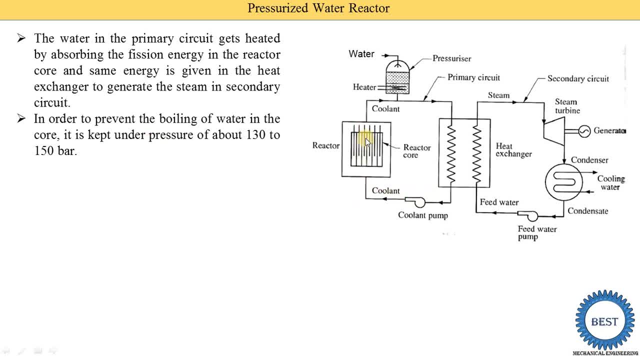 Means this coolant supply to this reactor with a pressure of 130 to 150 bars. Ok, So they are in a water state and this water is coming out from this coolant and it is supplied to heat exchangers So it help in absorbing the heat by water in a liquid state in the reactor. means due. 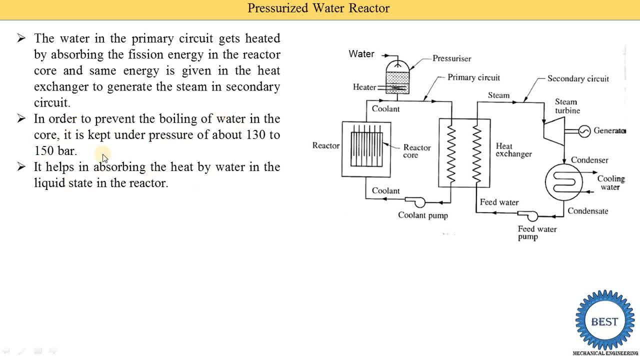 to this. high pressures means this high pressure is help to absorb the heat energy into liquid state. It is not convert into vapor state Because at the 130 or 150 bar The boiling temperature of the water is increased. Ok, At the atmosphere pressure the boiling point of the water is 100 degree. 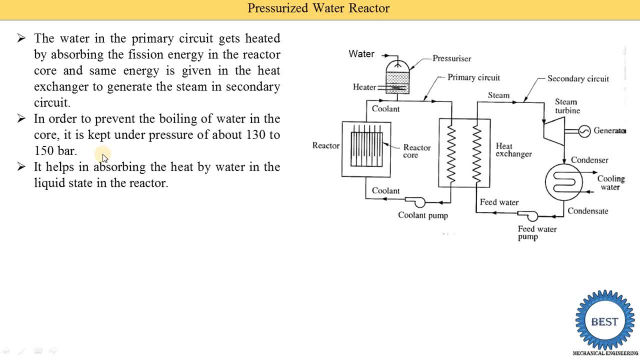 But here pressure is higher. that means boiling point temperature is also higher, Means its temperature are above the 200 degree centigrade. The steam produced in the secondary circuit is used in a conventional way in a steam power plant cycle, as shown in this figure. 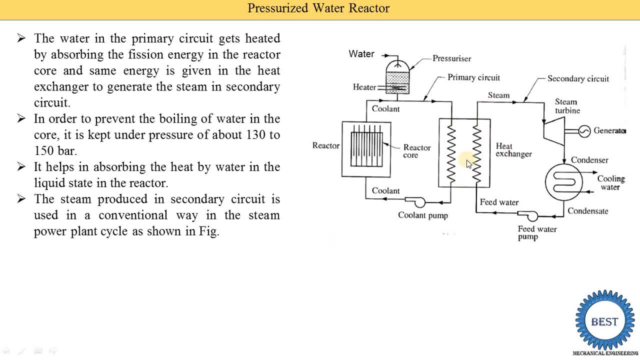 So here steam is generated in the secondary circuit in this heat exchangers. Ok, Even after circuit is same as the conventional steam power plant. means the as a Rankine cycle. Ok, So in a Rankine cycle after the boiler, or a steam generated by the boiler, it is supplied. 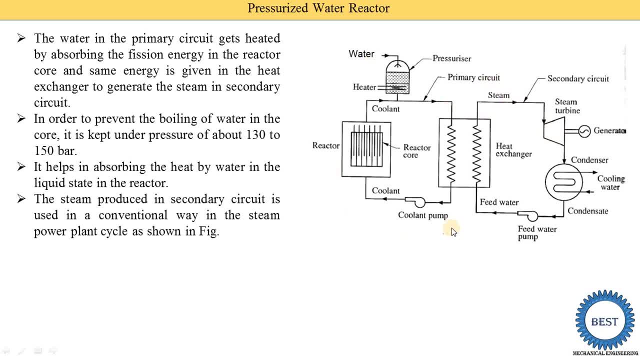 to turbines. Ok, So here steam is coming out from this reactor, means this is the component used. instance of this boiler: Ok, These reactors pressurizer heat exchangers. So this steam is supplied to this steam turbine in a steam turbine isentropic expansion process. 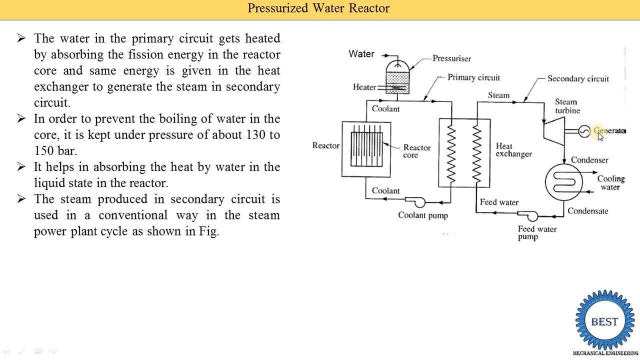 is carried out. Some work is produced by the steam turbines. This generator is running. This generator is runs by the steam turbine and electricity is produced. Then the steam coming out from the turbine is supplied to this condensers. In this condenser the steam is convert into the water. 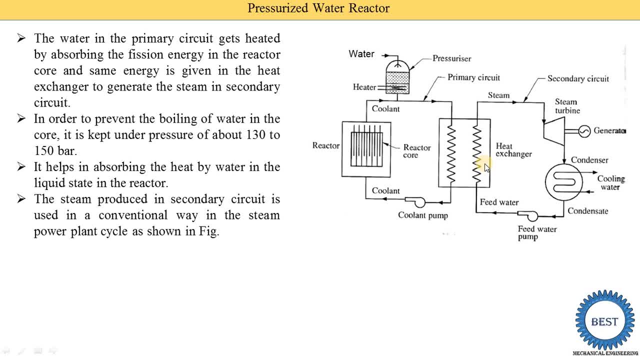 And then it is supplied to feed water pump and then again supplied to this heat exchanger. This way, the cycle is continuously run. The water coolant from the heat exchanger is recirculated to the reactor with the help of this coolant pump that we already discussed. 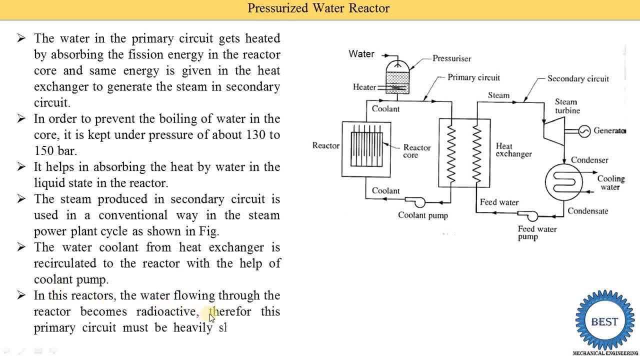 In this reactor. the water flowing through the reactors From radioactive means. water flowing through the reactor means from this part- Ok, The waters are radioactive. Therefore this primary circuit must be heavily sealed to protect the operator means this: we need to only seal to this primary portion. sealing of the secondary circuit is not required. 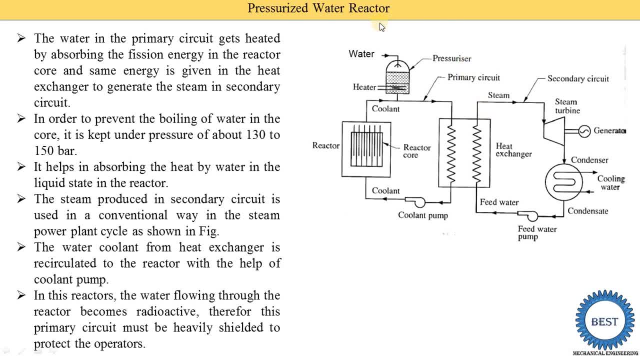 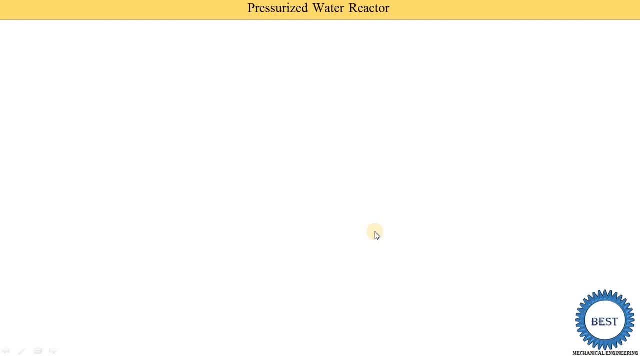 because here that is a indirect heat transfer, or takes place, So only primary circuit are shielded. Ok, Now we understand the advantages and disadvantages of this PWM. Ok, Before moving on that, I request to like the videos and subscribe my channels for watching. 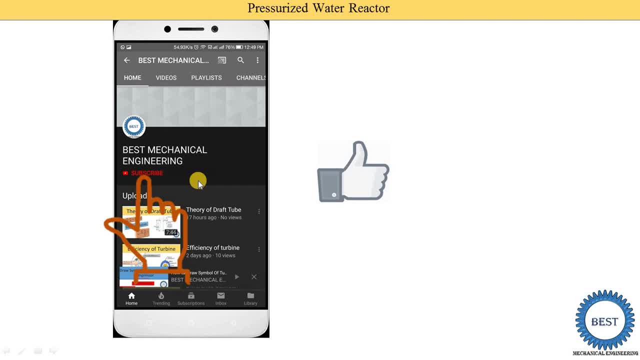 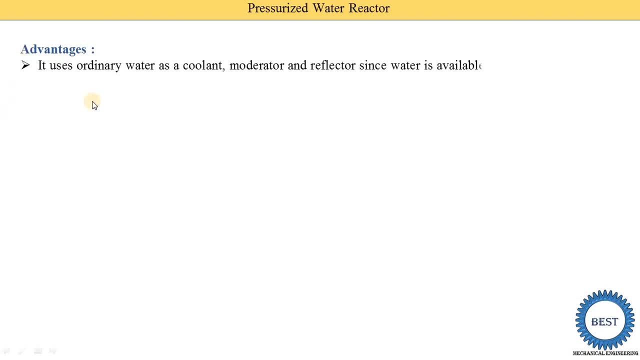 the more video related to the power plant engineering or other subject of this mechanical engineering. Now we understand the advantages. So in a PWM means pressurized water reactor, we use the ordinary water as a coolant, moderators and the reflector, since water is available in a large quantity and the free of cost. 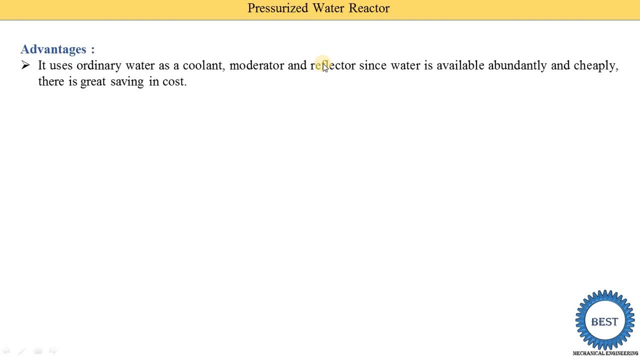 So there is a great saving in the cost because the water is available in large quantity and the free of cost we means we not need to pay any money for buying the ordinary waters. Ok, There is some processing cost, are there? only, The reactor is very compact and has high power density. 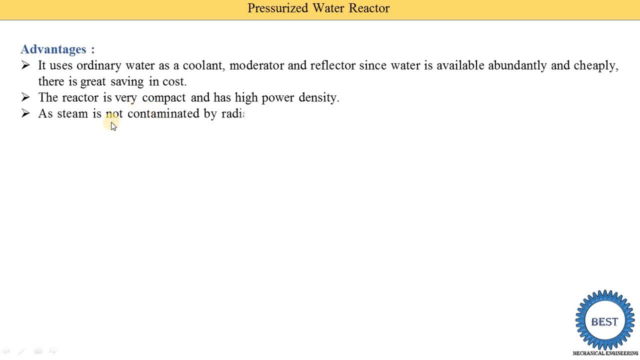 Compact means the size of this reactor are smaller. as steam is not contaminated by radiation, Inspection and maintenance of the turbine condenser and the feed pump is possible. Ok, So steam is produced in the secondary circuit. Steam is not produced in the primary circuits. 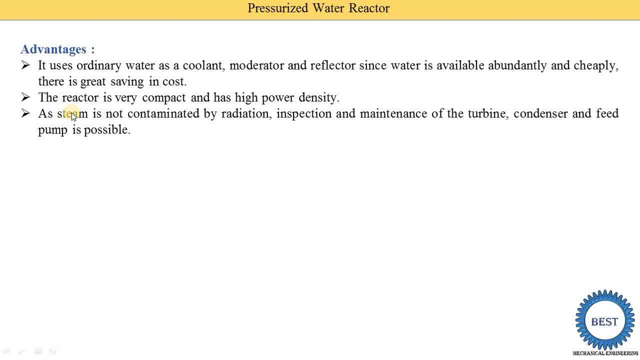 Ok, So inspections of the secondary circuit is easy. means the inspection either the maintenance of the turbine condenser and the feed pump is possible because they are the radiation free parts. Small number of control roads are required. means in the reactor the controller requirement is very high. 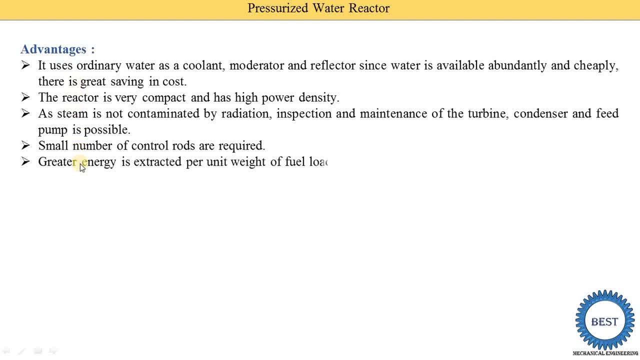 Ok, That is the small. Greater energy is extracted per unit weight of fuel. loaded means with compared to the fuel we can extract. the great energy means from the small quantity of the fuel we are extracting the great energy. Ok, So this is also the meaning of the high power density means from the smaller fuels we can. 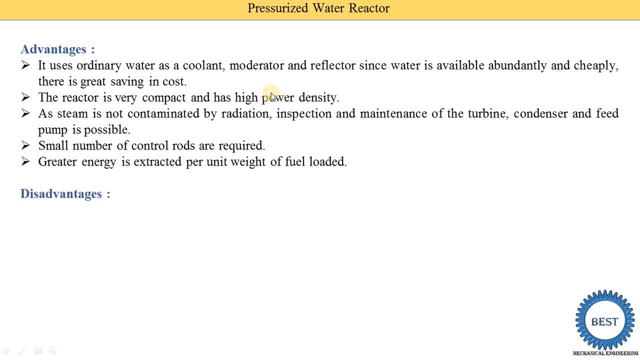 extract the more energy. Now, last topic is the disadvantages. First disadvantage: Its capital cost is high due to heavy and strong pressure, vessel is required in the primary circuits. Ok, So in a primary circuit the pressure is high, that is a 130 to 150 bar. 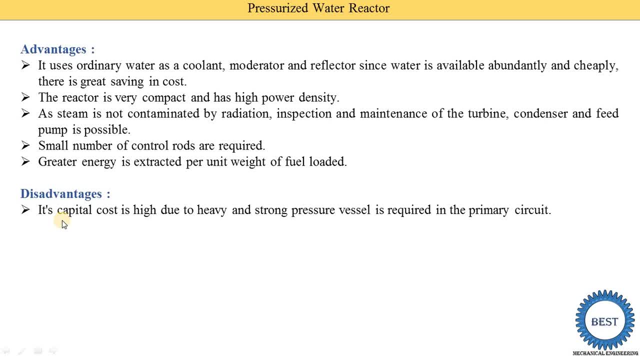 Ok, And we are need to completely seal the primary circuit because it is the radioactive parts. that is why the capital cost is increased. The thermodynamic efficiency of this plant is as low as 20 percent due to low pressure in the secondary circuit. So in the secondary circuit the pressure is low and due to that thermodynamic efficiency. 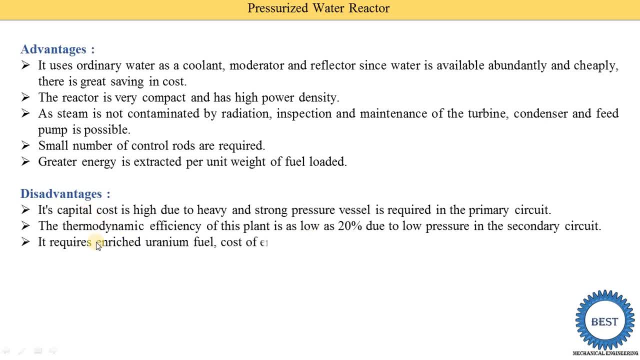 of the plant is low as 20 percent. Its require enriched uranium fuel, So cost of enriched uranium is high. Ok, So in a pressurized water reactor we are not use the natural uranium. Ok, That we already discussed in the first point.